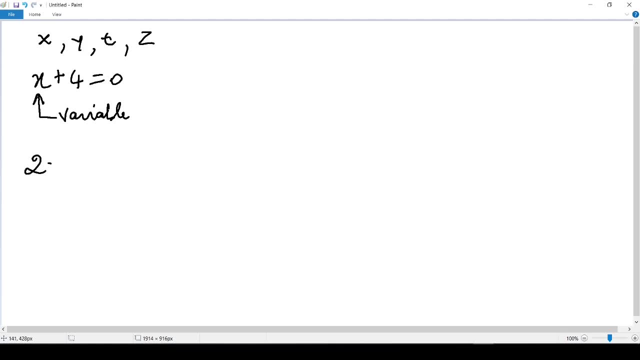 variable. so let's say 2x plus 1 for X, right? in this case our variable is X and we have 2x and equal x here. so thats 2x in our equation. the x is just repeated twice, but is still the same X, right? so our equation here still in one variable. 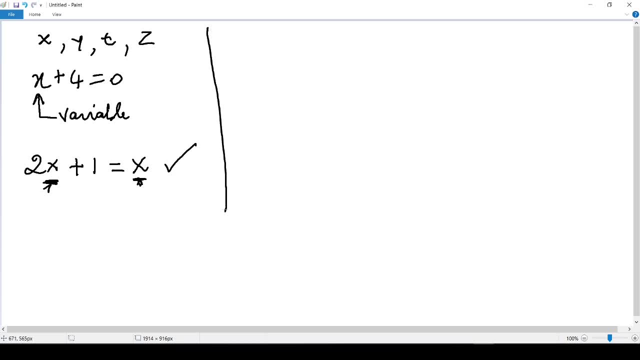 now let me ask you: is this position 2x plus y, equal to one equation in one variable? answer is no, because in this equation we have x and we have y and they are both different. x and y are different, they are not same. so in this case our equation is: 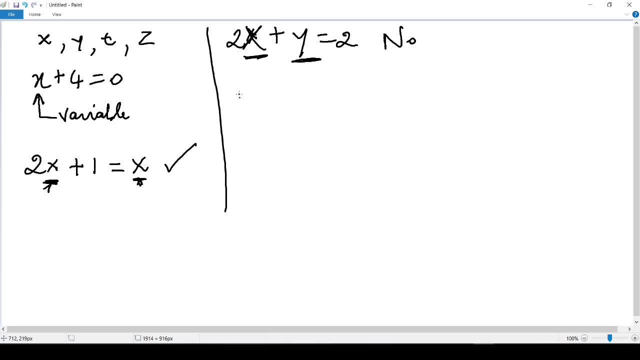 not in one variable. so what about 4x plus x equal to 1? the answer is yes, we have one variable. X, even though it is repeated, is still our X right, so we can have the same variable repeated many times in the equation, it is still an. 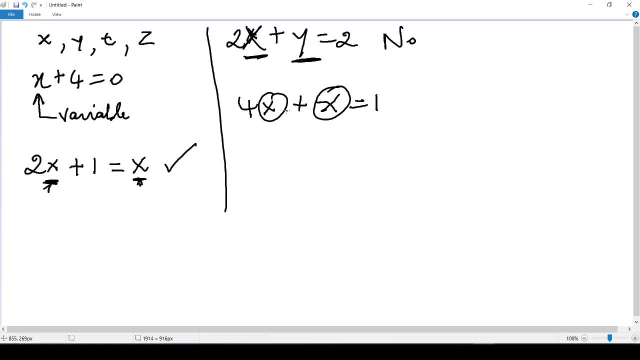 equation in one variable. good, now that we know what our equations are in one variable, let's solve some equations here. solving means finding the value of the variable in the equation. so if my variable in the equation is S, at the end of solving my equation I should have x equal to some. 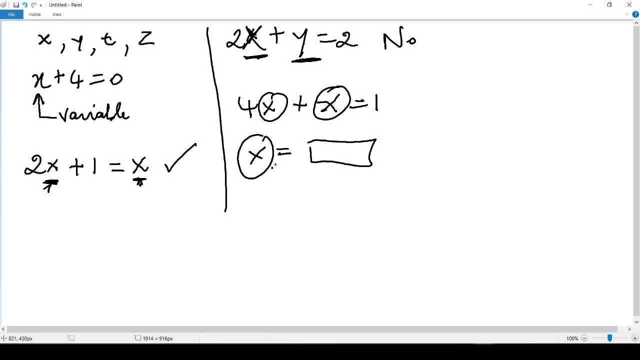 value right, X equal to some value. so that's our goal. if in my equation my variable is Y, at the end I should have y equal to some value. so let's say we want to solve y equal to some value. so let's say we want to solve y equal to some value. so let's say we want to solve y. 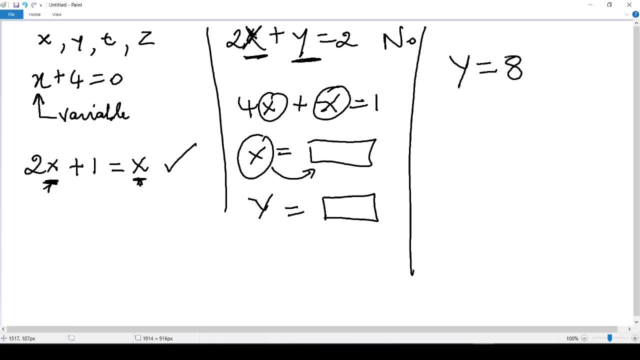 equal eight. the question is: solve y equal eight right, otherwise find the value of Y, Y. that's what the question says. if we say, solve y equal eight is find the value of y and, as we can see, the value of y is eight. so we don't need to do anything further for. 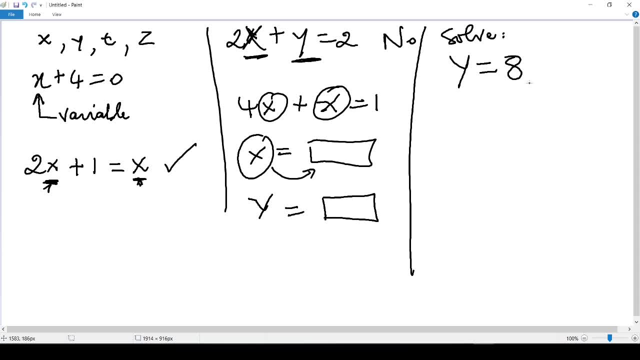 this equation. the equation is also the solution. so my solution is: y equal eight. so what about solving x equal to 10 y? so what about solving this x equal to 10 y? so we are just question. now, if there is knowing problem is solved, is the following question: solve sufferPrü потерper country. our equation in S 8 equally totals the value of y with the value of $8: 1, 2, 2, 3, 6. so what about solving x equal to 0? pahren of $8, 2, 3, 5, 4. here where we got to solve y equal to 20, our focuses to 0 and nяти. 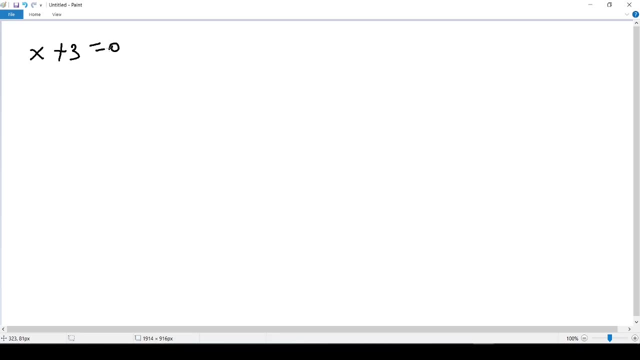 three equals zero. so in these equations our variable is X right. so at the, at the end, our results will give give us X equal to some value. so how to get from here to here with our value, we don't know yet. that's why we are solving so. 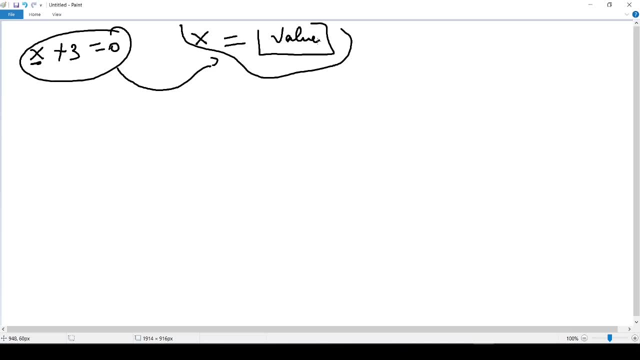 the first thing to think of is how to end up having X by itself on one side. and in order to achieve that, let me rewrite the equation here. we see that here we have 0 on the right and X plus 3 on the left. that means X is not by. 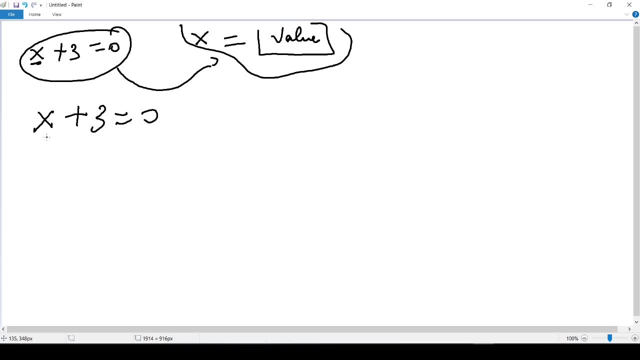 itself. the plus 3 is disturbing the X, if I can say that. so we will want to send our plus 3 to the other side in order to have our X by itself. so in order to do that, we add to our equation both side, the opposite of the. 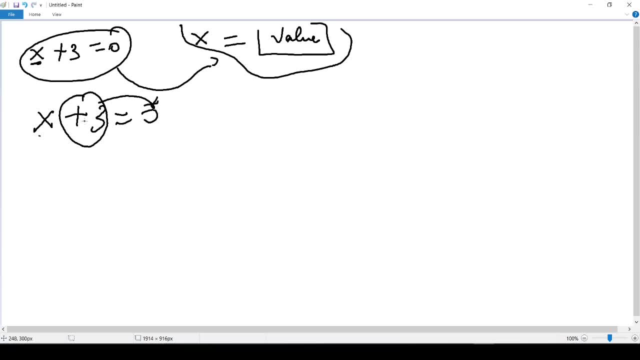 number that we want to move, and in this case the number that we want to move is 3, so as adding the opposite on both side remains adding negative 3 and negative 3 for each side of the equal sign and we perform our addition. so if I add X plus 19 is X, 3 plus minus 3 is 0, so they 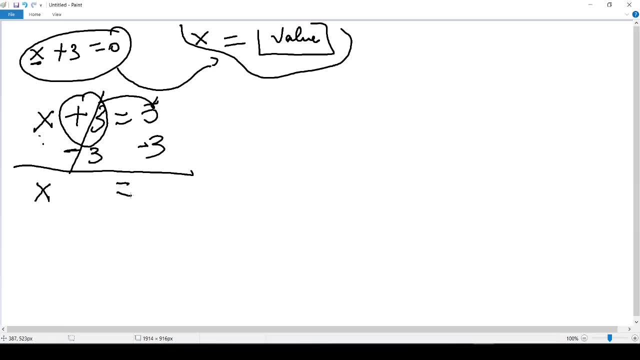 cancel. right, I'll bring my equal sign, and here I had: 0: 0 minus 3 is negative 3 and, as we can see, we have X by itself and negative 3 as the value of X. so we stop there because we don't have any further operation to do. X is, by itself, one side. 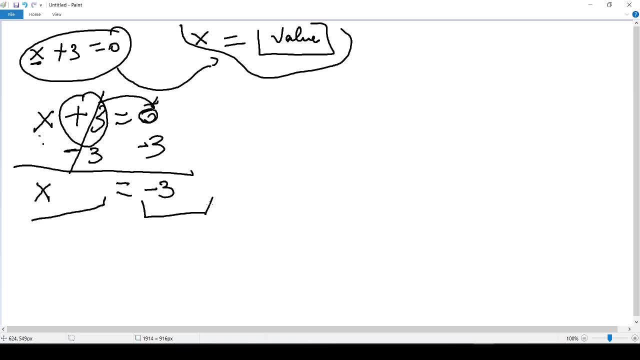 of the equal sign and all other values are on the other side. so X equal to negative. 3 is our final. so let's do another one. let's do 2 X 4 equal to 5, X plus 5. remember, we need to have X on one side and all other numbers on the other side, so doesn't. 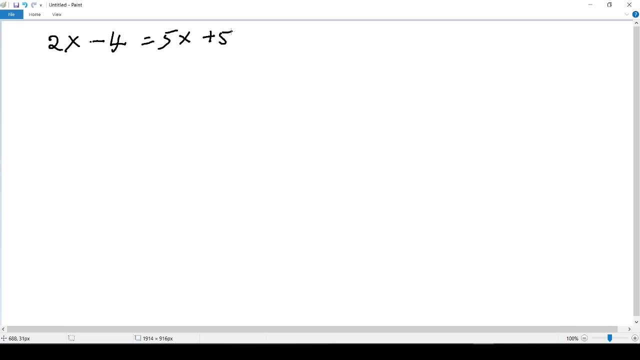 matter what side you want your X to be. in this case I would like my X to be to the left. so in order to do that, I will have to move there, this five X to the left, and to do that, this 5 X is positive. what I will do is add negative 5 X opposite. 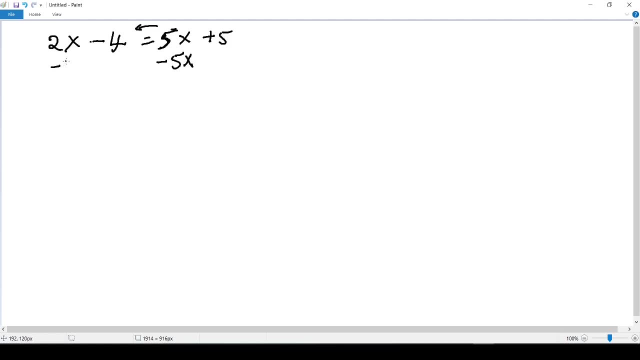 sign of what I want to do to both side of the equal soon. end all right and perform my addition. so 2x minus 5x is negative 3x. my negative 4: I'll bring it back here. it's still the same. my equal sign. I'll bring it down here. this 5x and negative 5x cancel because 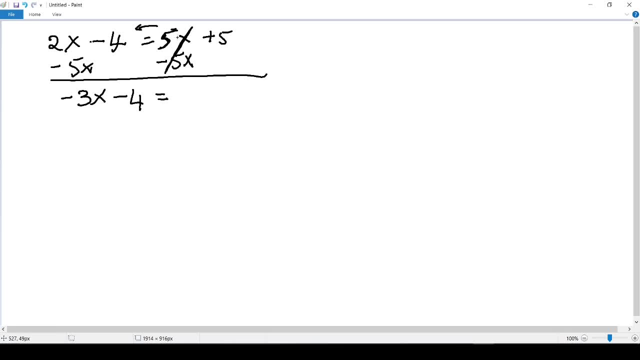 they are opposite sides, will give you 0, and that's why we use the opposite of whatever we want to move. and this 5, right there, plus 0, plus nothing equal to 5, right, are we done? no, why? because we see that this 4 doesn't have X, but is on the same side as negative 3x. 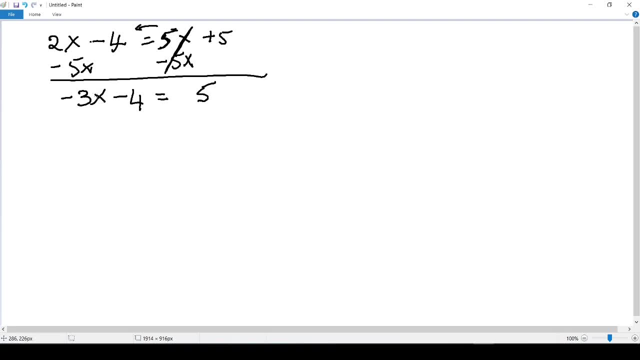 that's not our goal. our goal is to have X by itself on one side. all right, so the next step is to move this negative 4 to the other side of the equal sign. in order to do that, we will be adding 4 to both side. okay, so negative 3x. 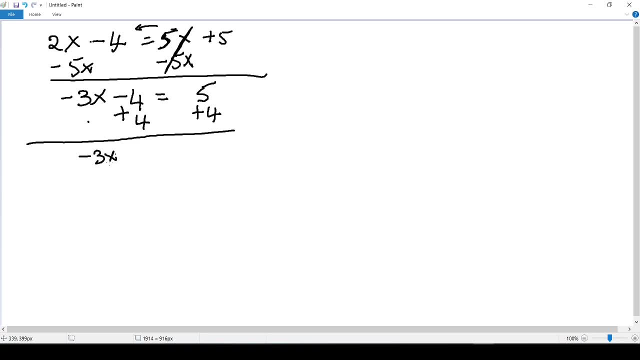 negative 3x. negative 3x plus nothing equal to negative 3x negative 4 plus 4. they cancel right. my equal sign is there and 5 plus 4 is equal to 9. are we done? no, because our goal still to have X equal to something. in this case, we have negative 3x equal. 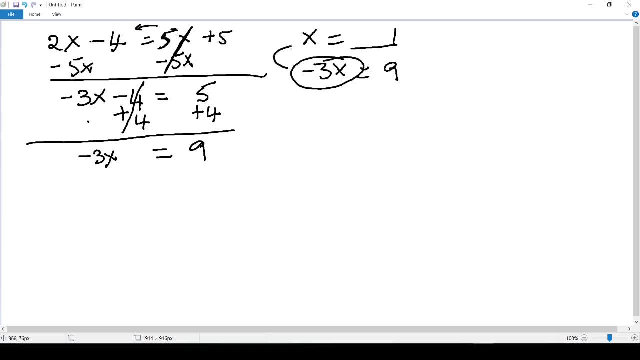 to 9. negative 3x is not X. so how to find X? we will divide by negative 3 in order to get rid of these negative 3s. we will divide our negative 3s by negative 3, each side, so negative 3, negative 3, so negative 3x divided by negative 3 will give me a: 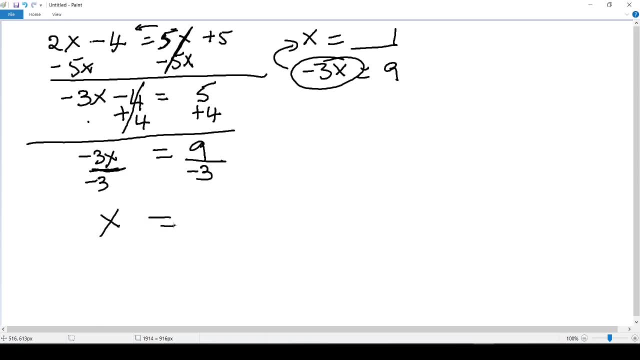 negative 3x right and 9 divided by negative 3 will give me negative 3. are we done? yes, why? because we end up having X by itself equal to negative 3 the value. so we stop there. that's our closer. another one let's solve to this: X plus 1. 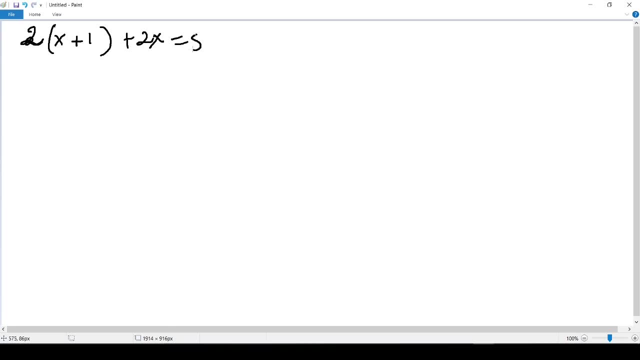 plus 2, X equal to 8. okay, here we introduce parentheses with some values inside. so what we do first is realize that this 2 is multiplying. this whole sets, right here, X plus 1. so the next step is to write our equation without a parentheses. so we will distribute the 2 inside our parentheses and get rid of. 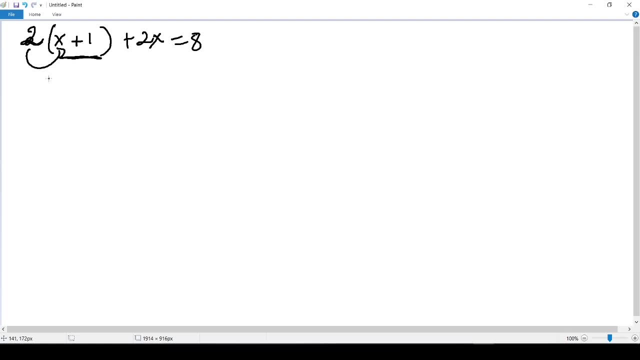 the parentheses. we will do: 2 times X, it's 2x, right and the same. 2 times 1 is 2 and in the middle we have the plus sign. we put our plus sign and we keep doing the rest, because these two doesn't affect the rest of our. 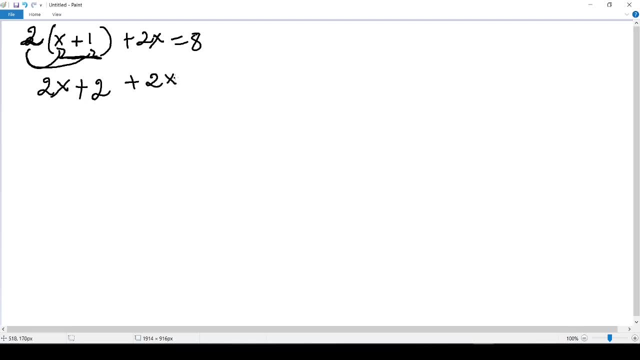 equation. so plus 2x equal to 8. okay, now we have our variable X and X here, two X's on the same side. so what we do is combine them, because they are like terms and they are on the same side. we will combine them. so we will combine these. 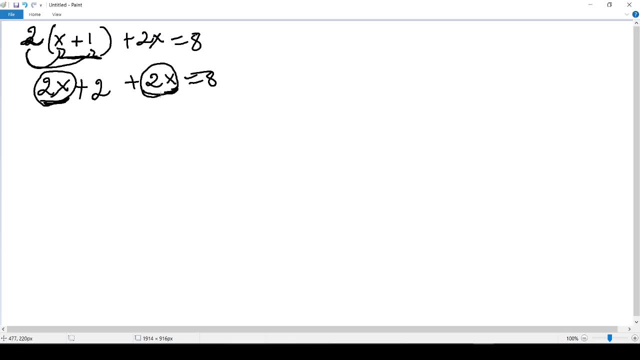 two X to these two X, and that should give us four X, and here we bring our 2 plus 2 and equal to 8. the next step is to move these two to the other side, because we want the X to be by itself. so what we do is add negative. 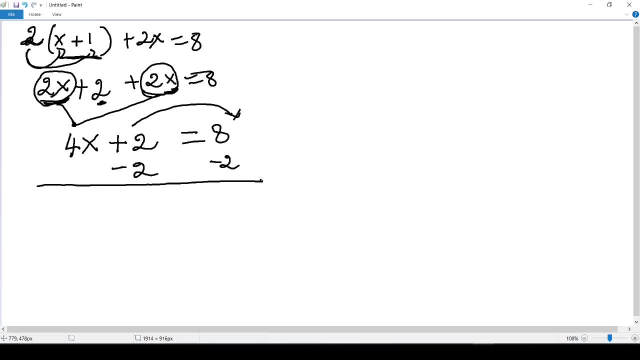 two negative, two to each side. we have four X here. these two cancel our equal sign: 8 minus 2, 6. okay, so we have four X, but we are looking for X. so what to do is divide the whole equation by 4, 4, 4. I want you to realize that we are not. 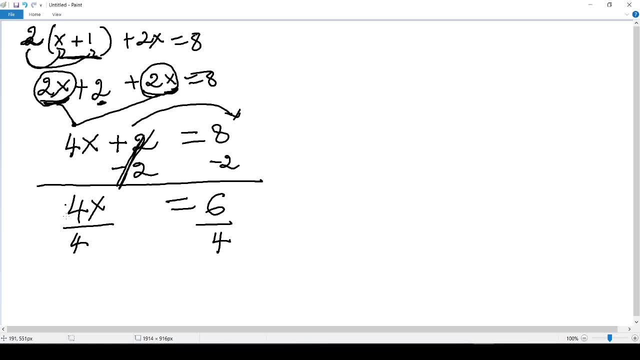 dividing by 4 X. we are only dividing by the coefficients and this will give you X equal to 6 over 4. you can reduce the equation and you will have X equal to 3 over 2. final answer: don't be afraid, because you find a fraction sometimes. 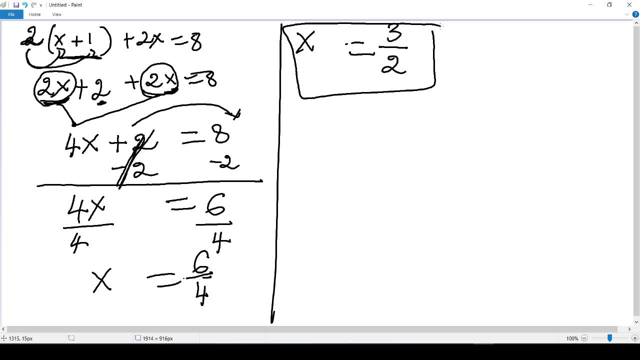 when we are solving our math problems and we end up half fraction and we start thinking: did I get it right, did I get it wrong? because it's just a fraction. a fraction is a number. so once you have a fraction, don't get confused about it, don't get scared about it. it can be your answer. okay, yeah, sometimes solving the 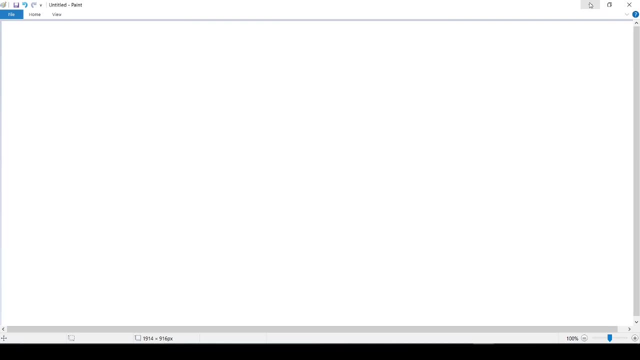 linear equation in one variable doesn't return exactly one solution. that's Much less than 0.5 USD. so the following example will show us a case when we don't have one solution as an answer. so let's solve 4X minus 6, equal to two parentheses, two X. 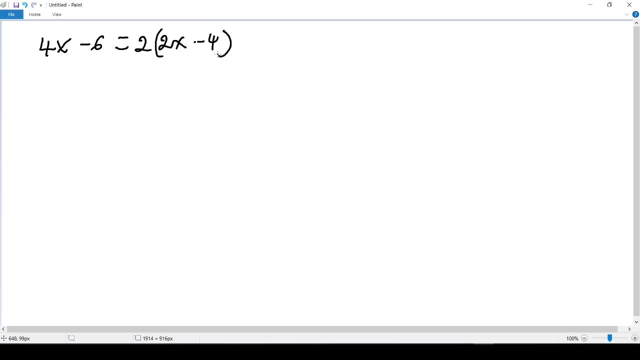 minus 4 plus 2. okay, so what we do first is take care of the parentheses, so we will distribute the two inside and then get rid of the parentheses, so we will have 4x minus 6, equal to 2 times 2x is. 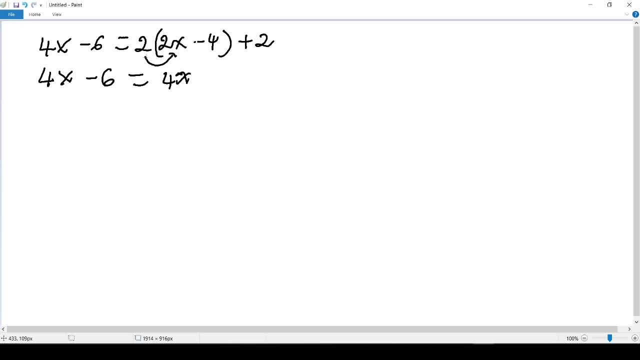 4x, 2 times negative. 4 is negative 8. right, and now plus 2. okay, let's combine like terms whenever we can combine them. here we have negative 8 and 2, so we will combine them, so that will give us 4x minus. 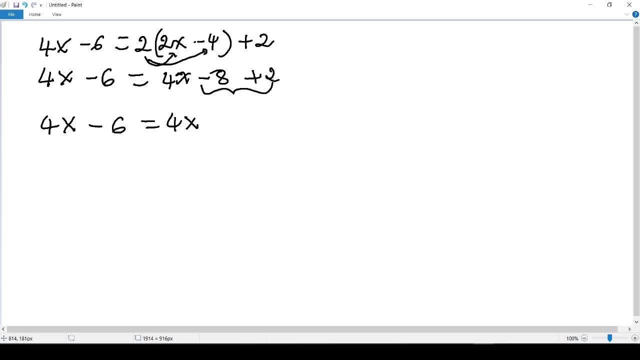 6 equal to 4x. negative 8 plus 2 is negative 6. okay, here we have to have X's on the same side and all other value to the other side. I choose to send my 4x, this 4x, to the other side. so what will I do? I will do. 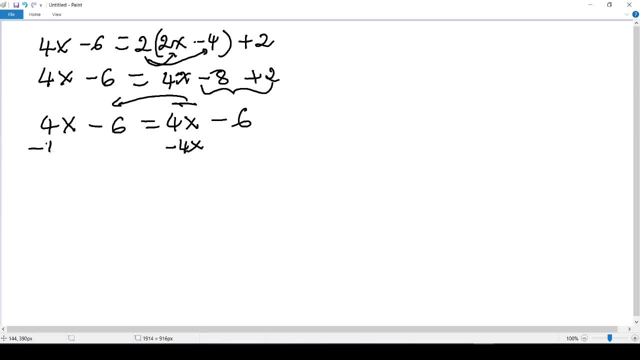 negative 4x, negative 4x from this negative side, right. and then I will add: then what we see is negative 4x and negative 4x cancel. I have negative 6 is equal difference in this 4x cancel. I have negative 6 right there, so I end up having negative 6 equal to negative 6.. 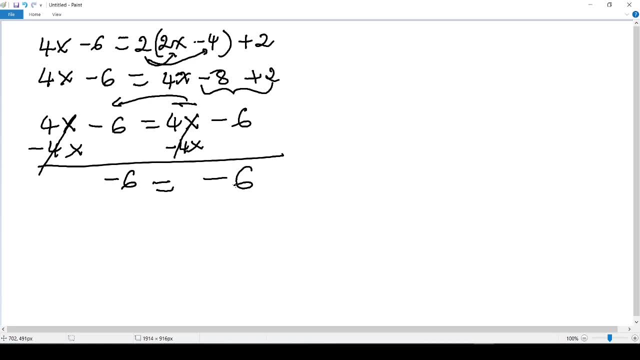 before I continue, look at this. in this case, I choose to move my 4x first. okay, I will rewrite it as 4x minus 6, equal to 4x minus 6. I'm just rewriting this right there, and in this case I will be moving my negative 6 to this side, so I'll be. 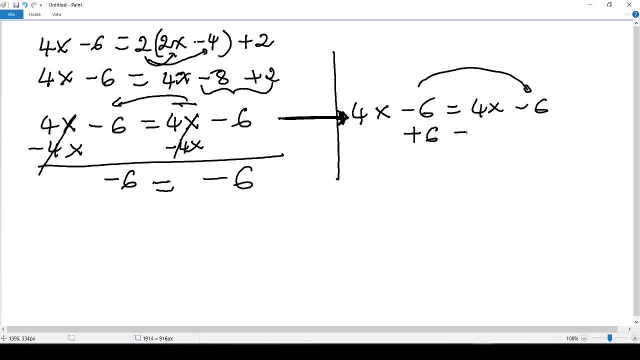 adding 6 to both side and I'll be performing my addition. I have 4x right here. this 6 and negative 6 cancel equal to this 4x. 4x is right there and this negative 6 and 6 cancel. so, based on what I move, 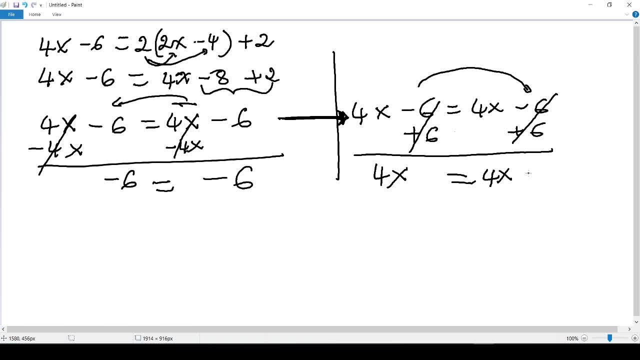 first. I have different result. alright, but what we realize is negative 6 equal to negative 6. my variable disappears. there is no problem there. here I have. so 2 x is divided by 6. so in myaz simulation we will write negative 6. Следdid, I forgot to add in the 4 and I use negative 6. I have Agora. I have negative 6. 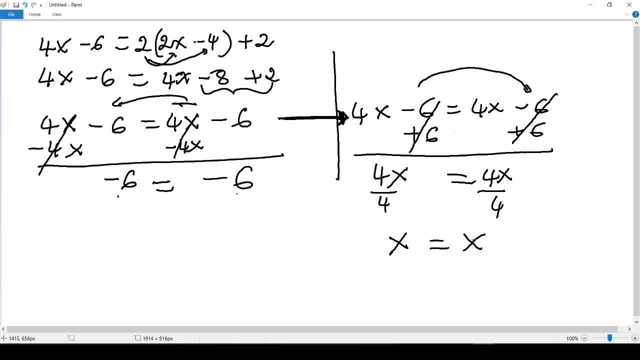 equal to negative 6. negative 6 is inside, so my mod Yani this: and negative 6 is inside, so let's just count this all. so negative 6. for me this is going to be 9x, which is mathematically is true. in this case, I have X equal X. 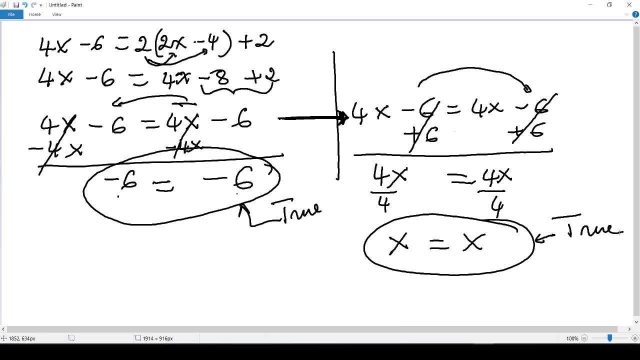 mathematically is true. X is a variable. that means if I put a number here, I should put the same number here. if I put negative 6 here, I should put negative 6 here. if I put 7 here, I should put 7 here. so negative 6 equal to negative 6, 7 equal. 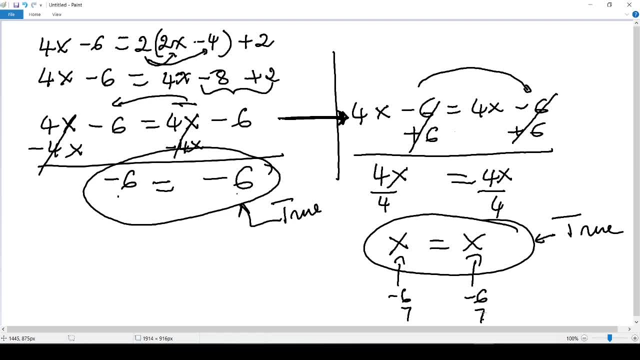 to 7. so once, after solving an equation in one variable, you end up having this kind of solution, where they are true, very important, have to confirm that whatever you have at end is true. then we can conclude saying that all real numbers are solution to our equations. 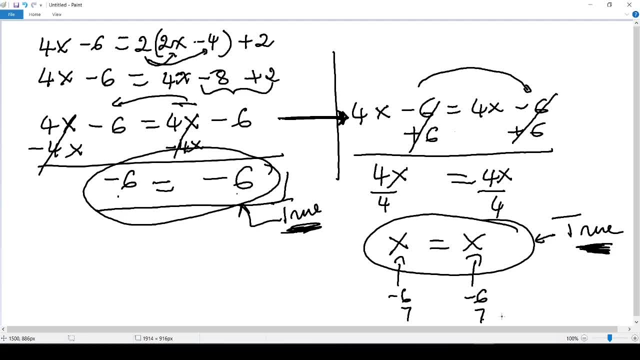 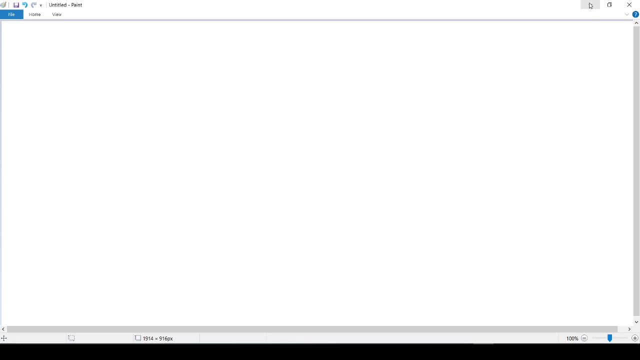 right, all real numbers are solution to our equations. so once you have this setup you can give that conclusions: all real numbers are solutions. something solving linear equation in one variable returns no solutions. so let's see that by solving this equation, 4x minus 6 equal to 2 to X minus 4, so we have 4x. 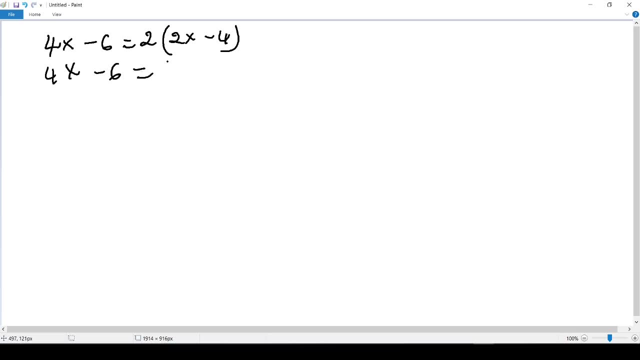 minus 6, equal to we distribute the 2 right. there we have 4x, this minus 8. so I will choose to move my 4x from the right to the left. so I will be subtracting 4x on both side and I realize that this console I have negative 6, equal to this. 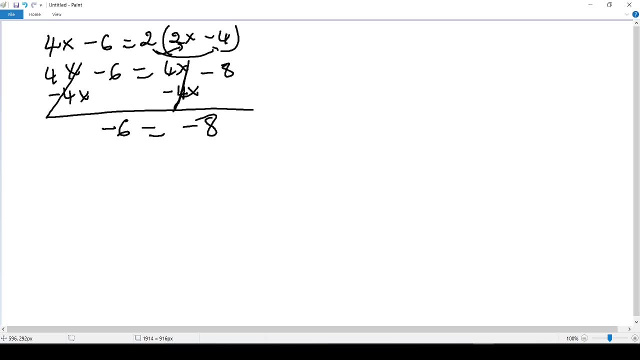 console and negative 8. in this case, negative 6 equal to negative 8, which is not true, so not true. or I can put false, so not true, or I can put false. so in case my result looks like this and is false when I say look like this, it. 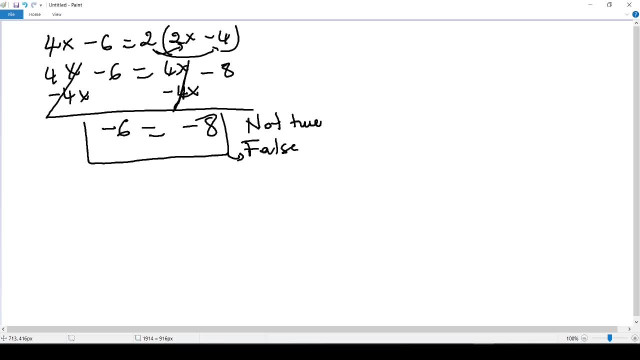 so, in case my result looks like this and is false. when I say look like this, it doesn't mean always have negative 6 and negative 8, but when I end up having two difference number, each side of equal sign and it doesn't mathematically make. 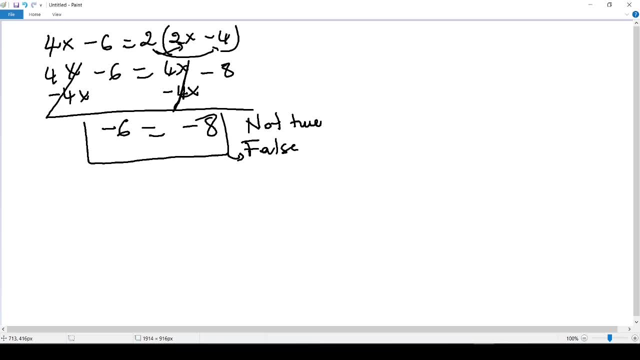 any sense that means it is false right. any sense that means it is false, right. so once you have false, that means you have no solution to your equation and the result is no solution. that's what you should write as result after solving this equation, and we call this type of equation contradiction. so that's how we. 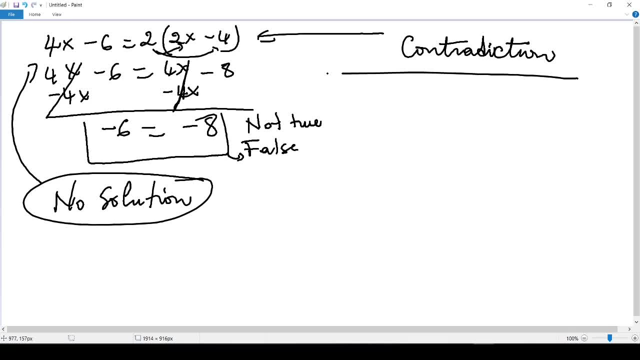 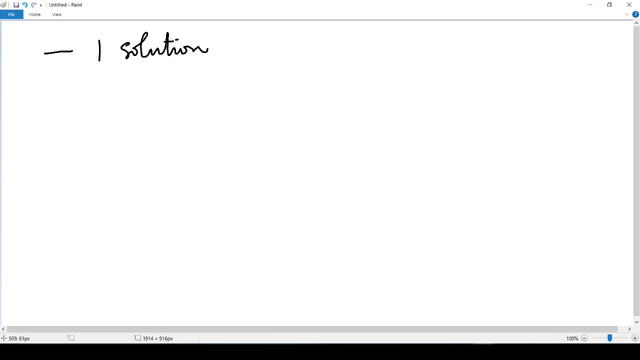 call this equation, say that it is a contradiction. in summary, solving linear equations in one variable can return three type of solution right. so first, the equation can have one solution or the equation has no solutions and we call it contradiction. and third, all real number are solutions, so all real